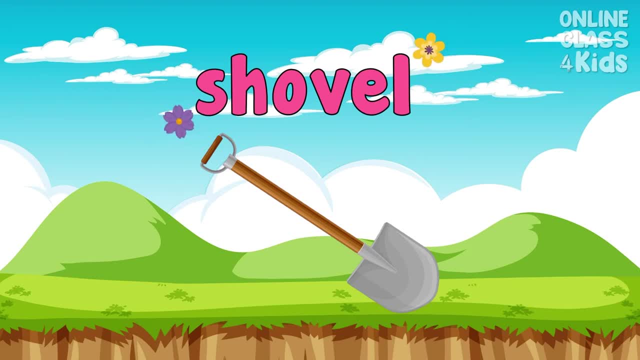 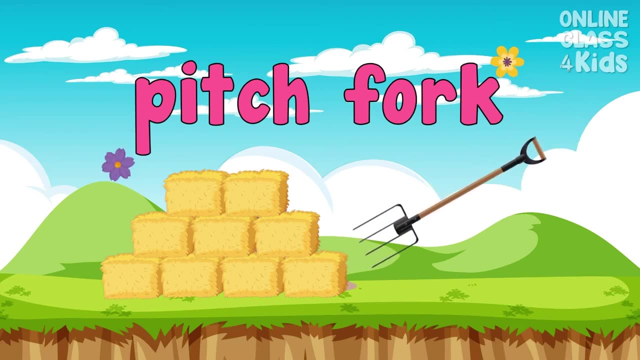 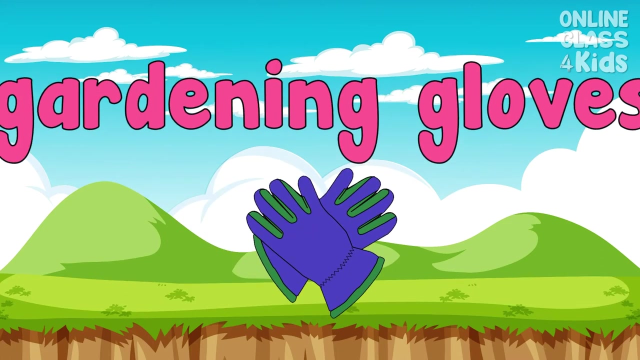 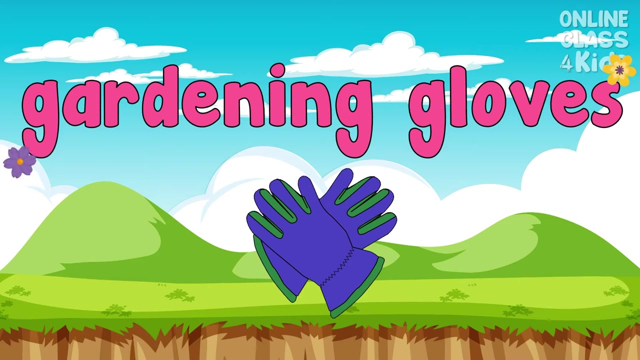 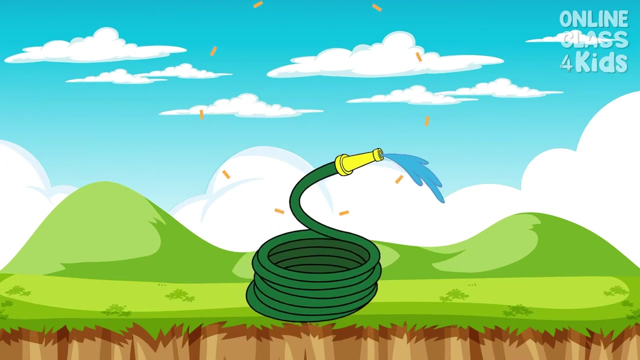 Shovel Say shovel. This pitchfork could be used to lift hay- Say pitchfork. When working in the garden, these gardening gloves are worn for safety. Gardening gloves Say gardening gloves. The plants are watered using this garden hose. 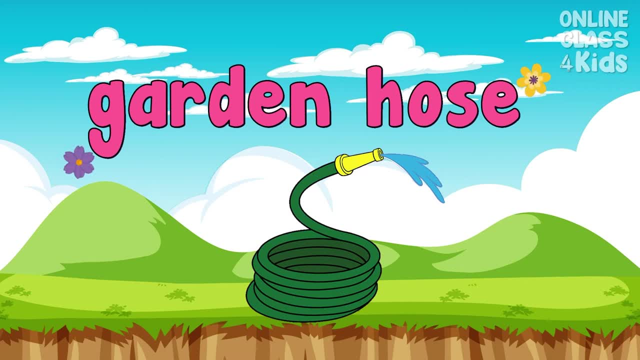 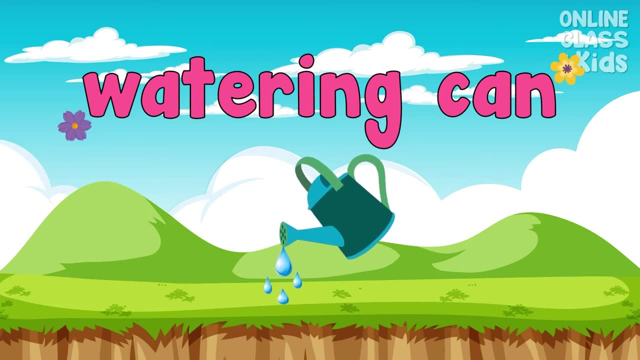 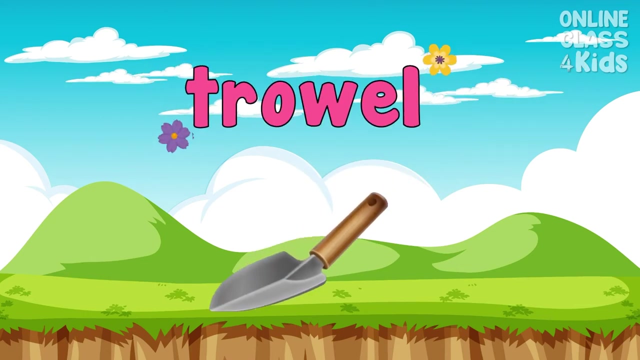 Say garden hose. This small container may be used to water plants by hand If you don't have a water hose. say watering can Again, watering can Use this tool to move or lift plants. Trowel, Say trowel. 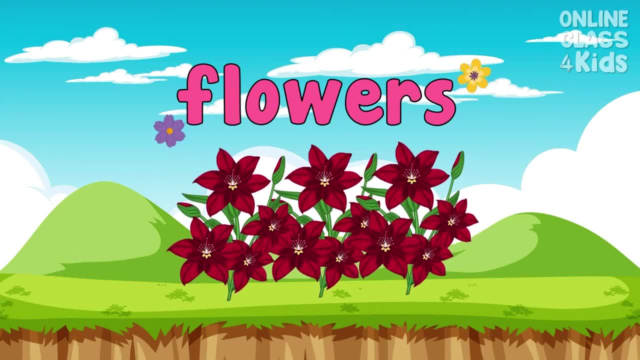 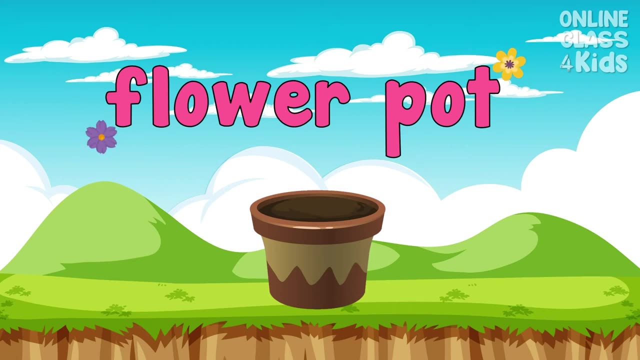 Wow. These beautiful flowers come in all sorts of colors and have a lovely scent. Say flower, Say flower Flowers. Some flowers are placed in a container called flowerpot. Say flowerpot, Say flowerpot. The gardener sweeps dirt or trash using a broomstick. 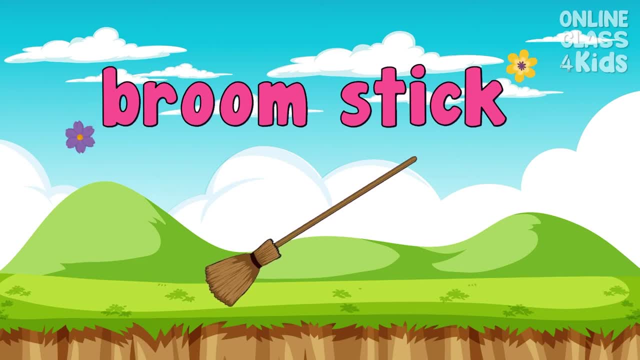 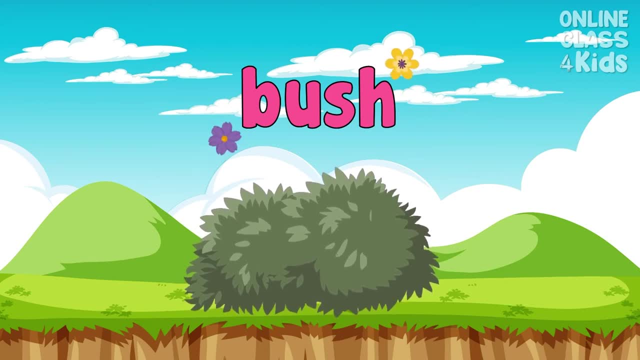 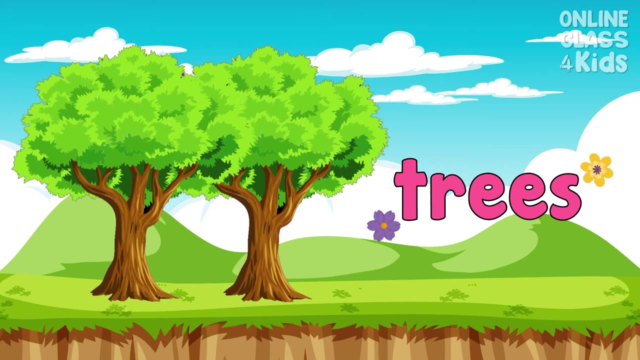 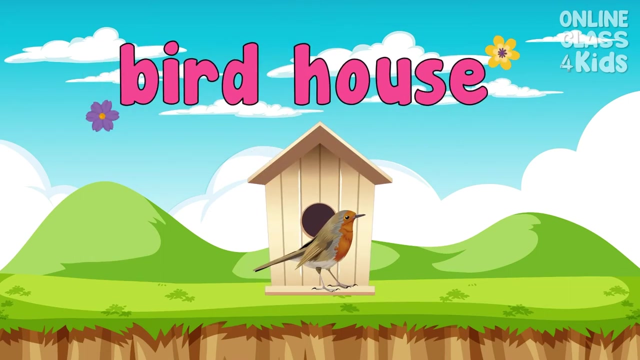 is smaller than a tree and has a lot of branches. say bush, again bush. aside from the flowers and bush, there are lots of trees too. say trees. this is amazing. this is called birdhouse, a small house as a place for a bird to build its nest. say birdhouse. 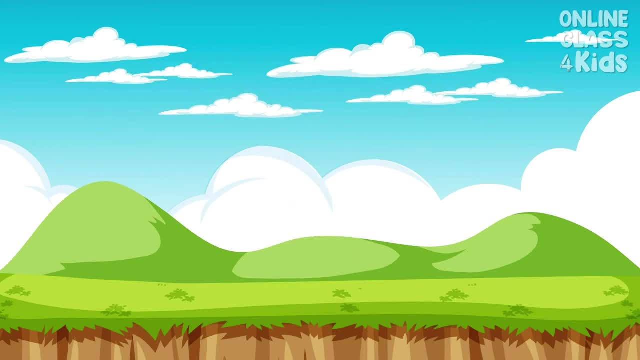 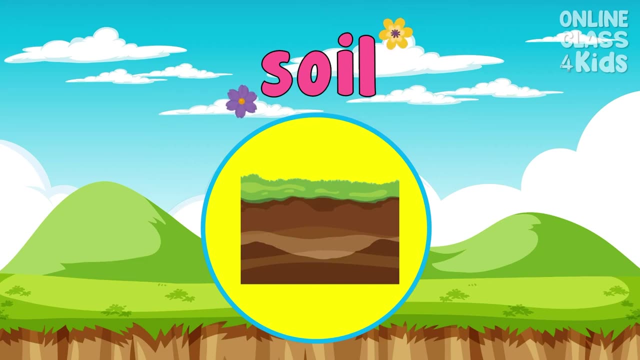 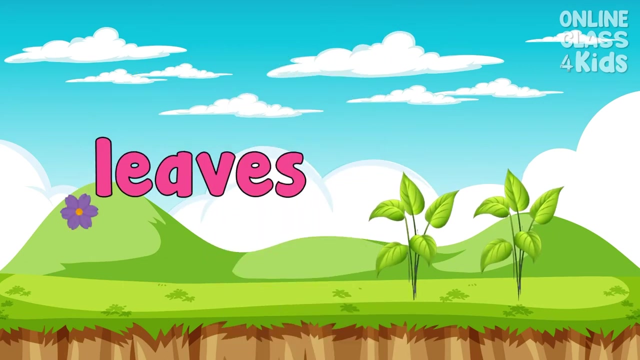 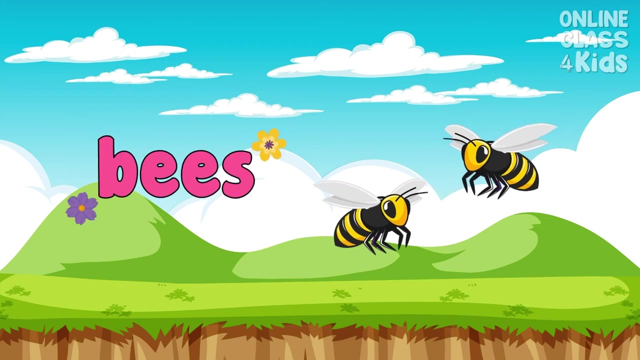 don't forget: you need soil to plant and grow trees. soil say soil. take a look at these luscious of green leaves growing from tree stems and branches say leaves. be careful of bees. they might sting, say bees earthworms. these are among the garden's most. 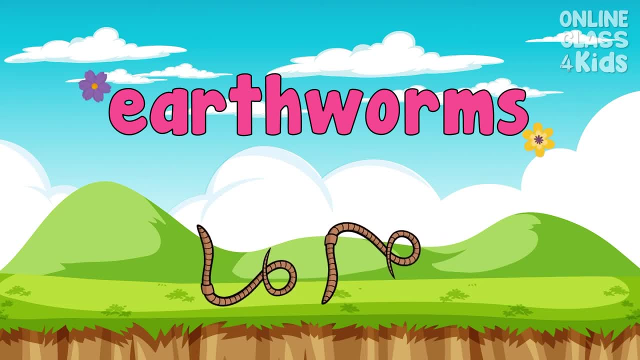 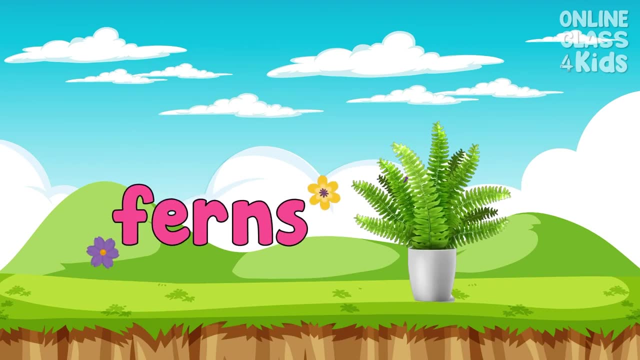 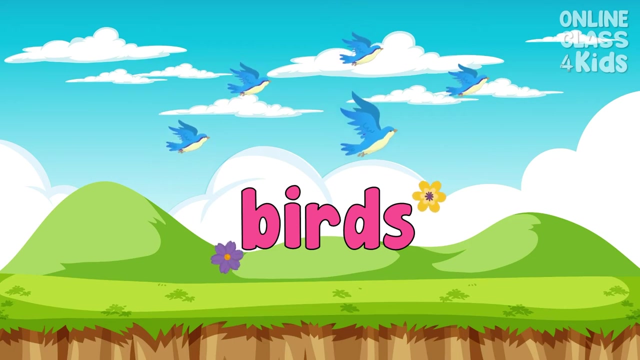 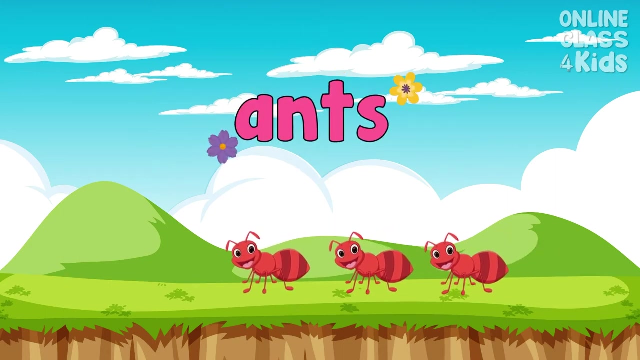 hard-working creatures, say earthworms. these green leaves shaped like feathers are called ferns, say firms. there are different birds around, say birds, say birds. these are flowers, very diverse. they are fennel. these are natural plants and they can grow in good shape. so garden has lots of ants, say ants. this tiny animal has a soft body and a spiral. 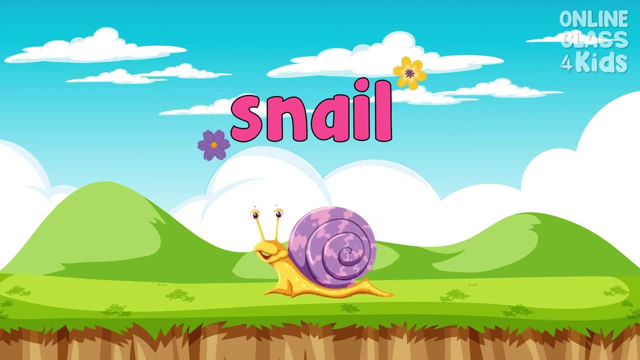 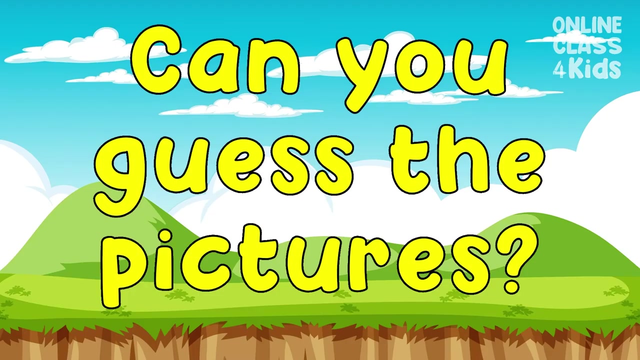 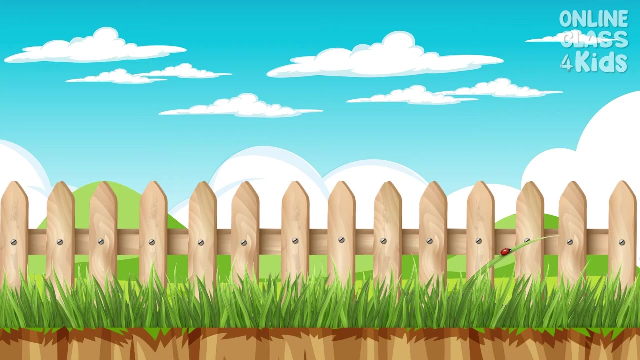 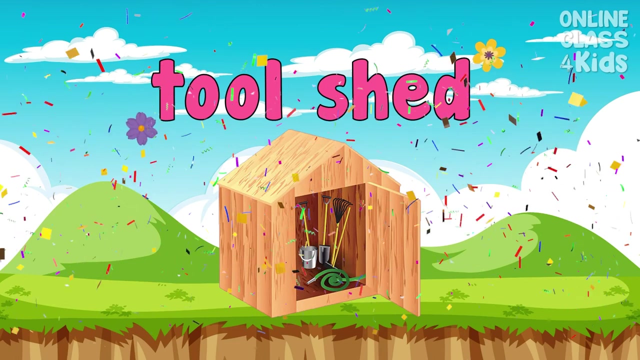 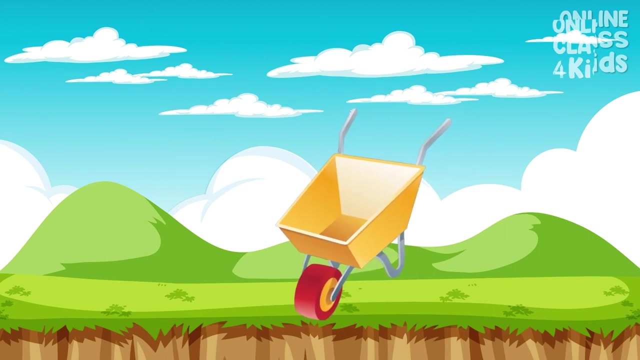 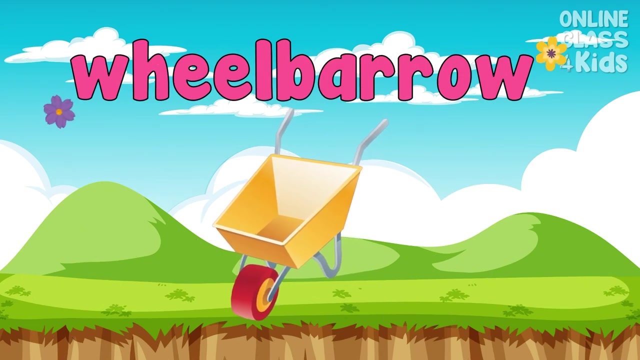 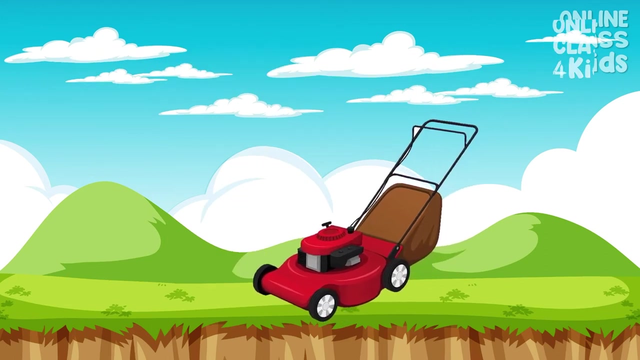 shell. you may see it on the ground, say: snail again, snail. now let's review what we have learned for today. can you guess the picture? yes, it's a fence. good job, that's a tool shed. well done. it's a wheelbarrow, correct, lawnmower. 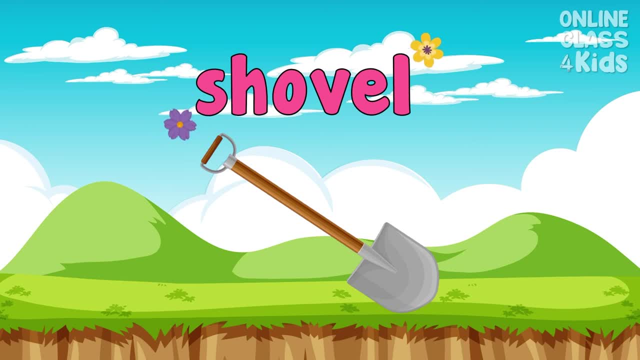 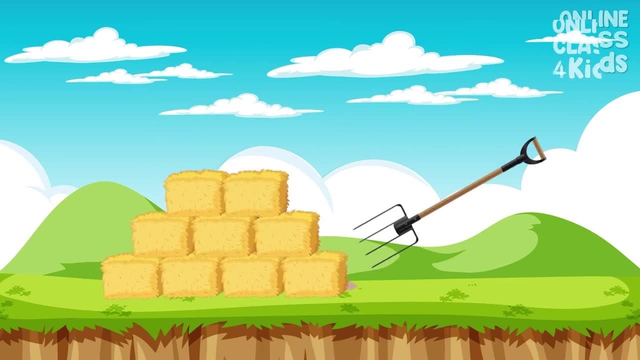 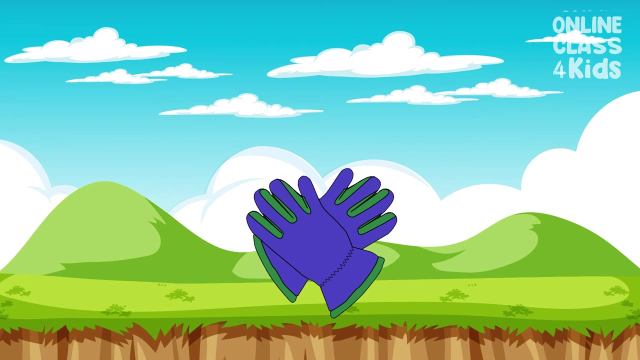 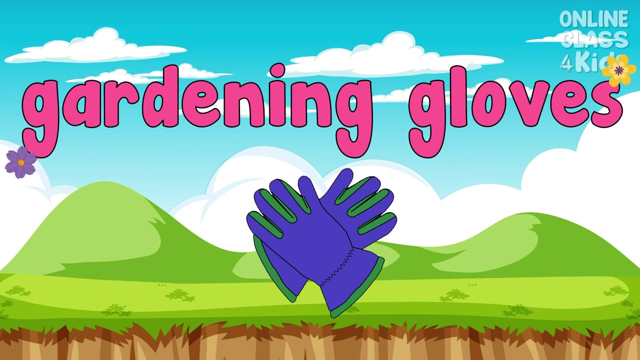 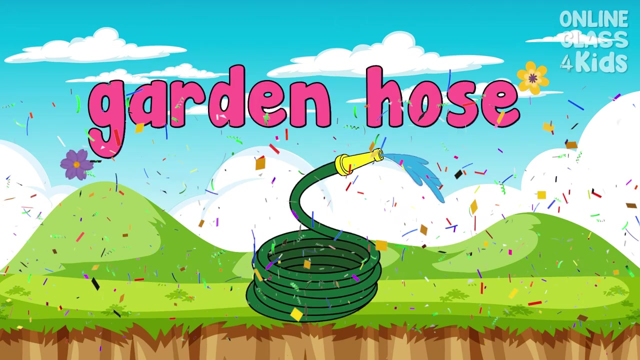 circle scarb, gorgeous, serves as trunk or drill. yes, it's a travel approved. nice research. what we have had a fun time with the. what we have had a fun time with the. this is really cool, guys. that's it. let's is our video Very good, It's a garden hose. 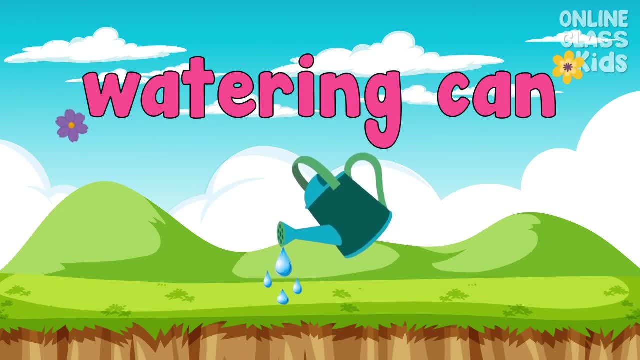 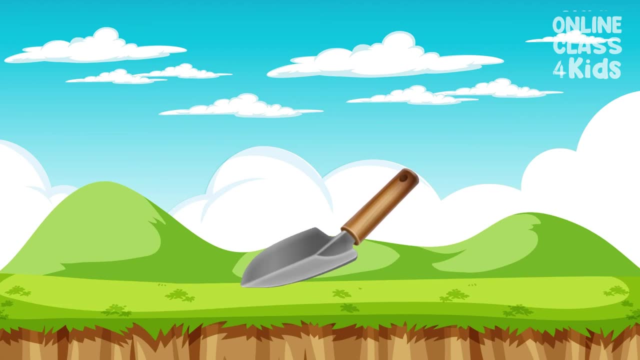 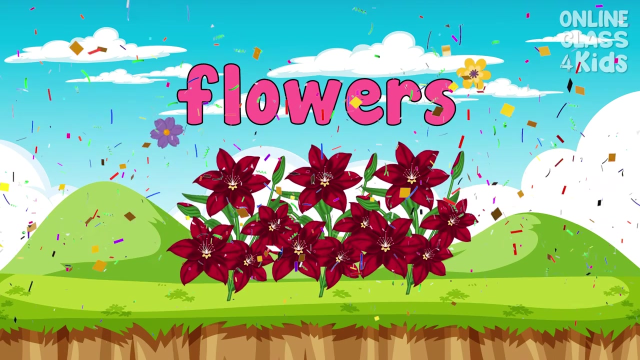 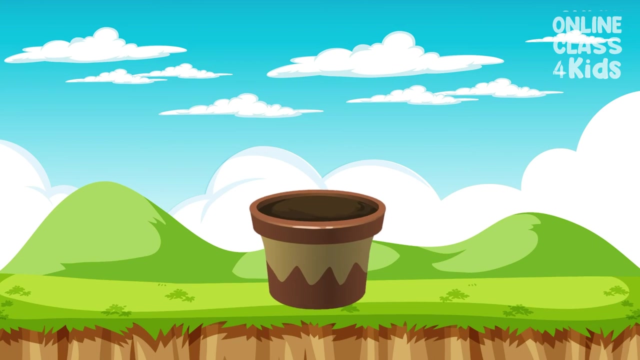 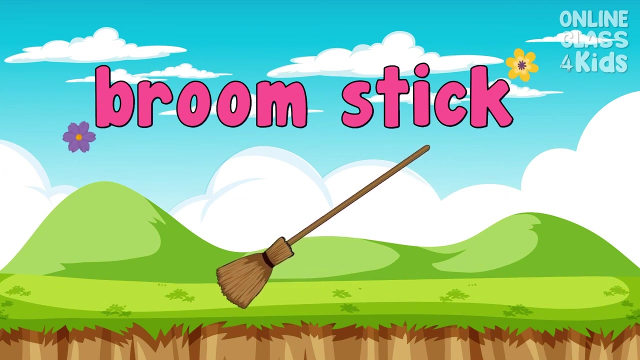 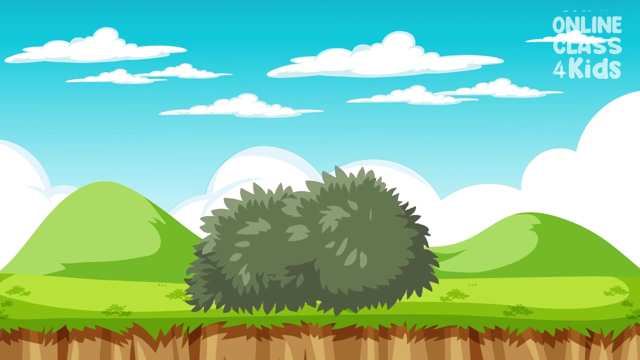 Excellent, It's a watering can. Congratulations. It's a trowel. You're right, Those are flowers. Yes, It's a flower. It's called flower pot. You got it right. That's a broomstick. Exactly, It's a bush. 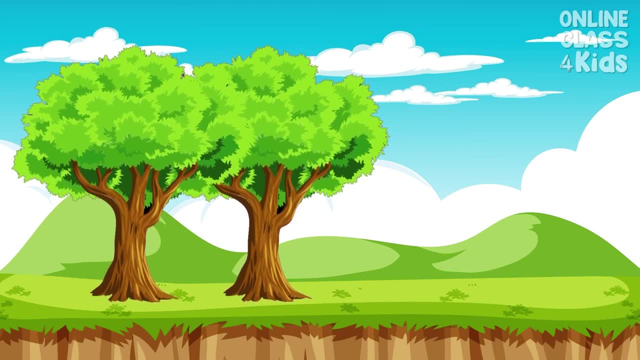 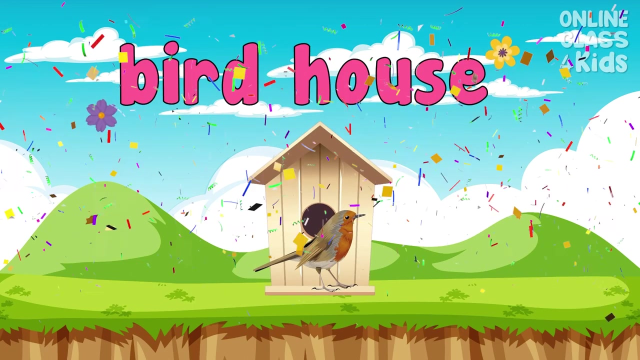 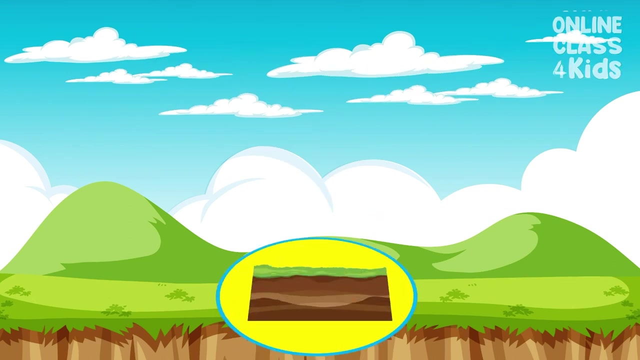 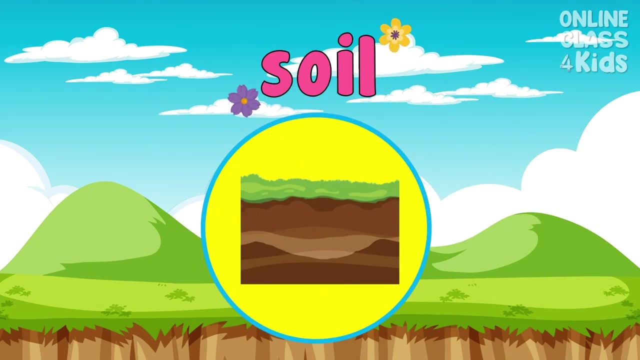 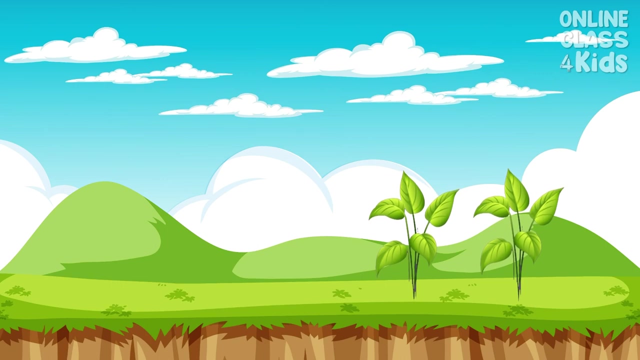 You got it right. That's a broomstick. Bingo. Those are trees. Yes, It's a birdhouse. Wonderful, That's a soil. Yes, You're right, Those are leaves. Nice one. Those are bees. You got it right. That's a bill.